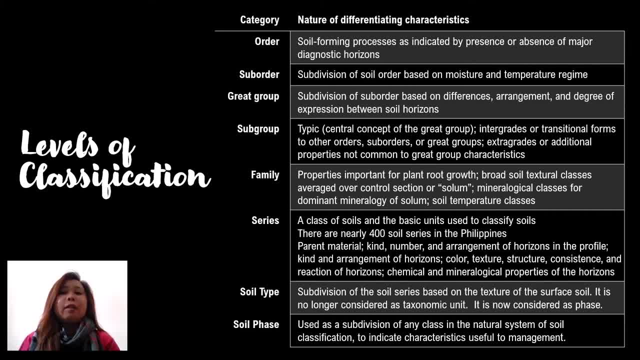 later on, as we proceed in this discussion, we will discuss one by one all those 12 soil orders, while suborder is the subdivision of soil order based on moisture and temperature regime. so later on we all we will also discuss the different suborders under the 12 soil orders. great group. 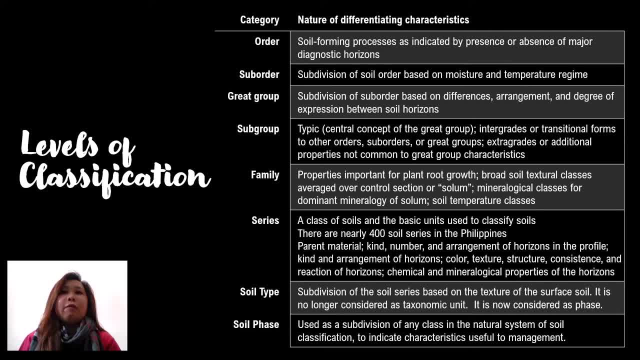 is the subdivision of suborder based on differences, arrangement and degree of expression between soil horizon. under the great group we have the subgroup. it is typic or the central concept of the great group integrates or transitional forms to other orders, suborders or rate groups. it could have extra grades or additional properties not common to great group characteristics. 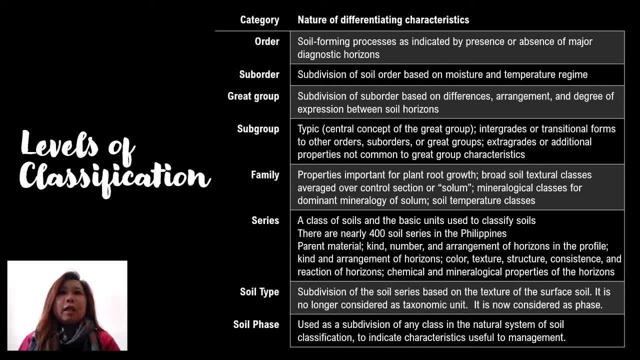 family. the nature of differentiating characteristic of family is that the properties important for plant root coat, broad soil texture classes, average over control section or solo, and mineralogical classes for dominant mineralogy of solum and soil temperature classes are those factors that are being considered in differentiating the characteristics of family. 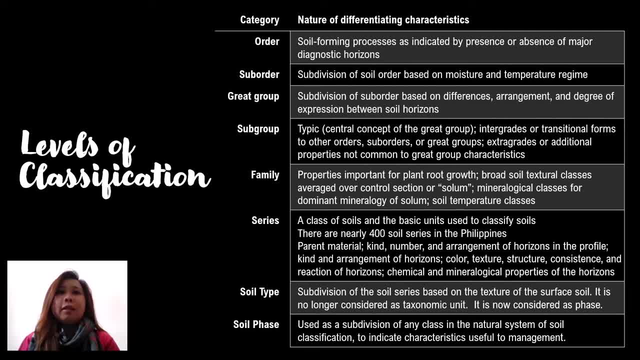 for series. series is a class of soils, of soil, size星 i, of species exploration, morteiro pineana, and the basic units used to classify swiss. there are nearly 400 solutions in the philippines. the parent material, such as the kind, number and arrangement of horizons in the profile, the kind and arrangement of horizons, color, textures. 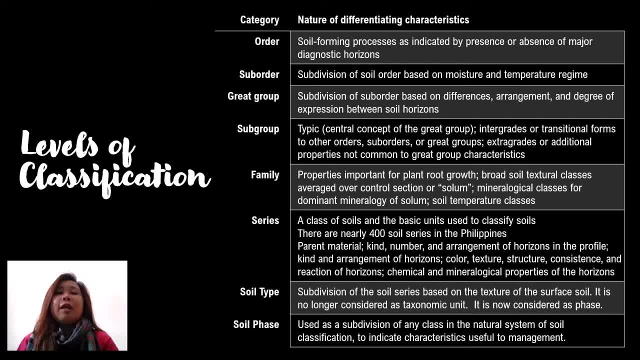 structure, consistence and reaction of horizons. chemical and mineralogy. mineralogical properties of horizons are being considered in classifying some engineer column for these properties. hvis case here: different soil series For soil type. it is the subdivision of the soil series based on the 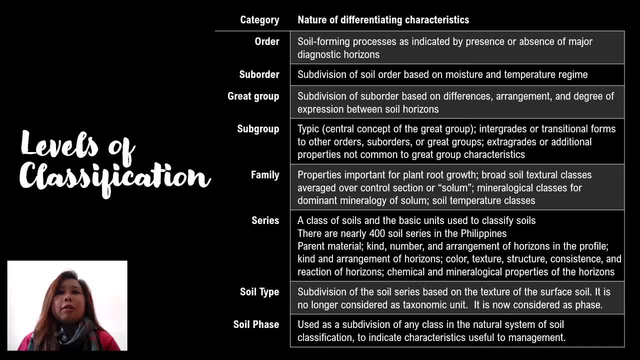 texture of the surface soil. It is no longer considered as a taxonomic unit. It is now considered as a phase Soil phase is used as a subdivision of any class in the natural system of soil classification. that is, to indicate characteristics useful to management. So let's 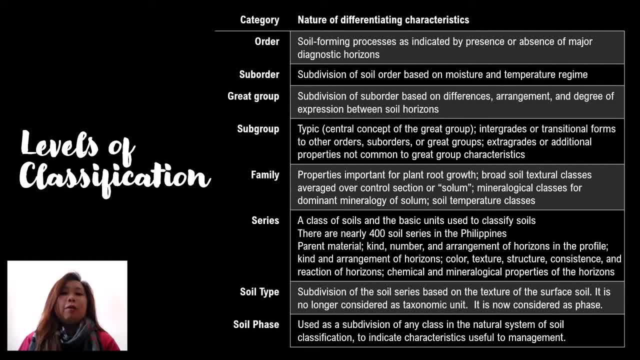 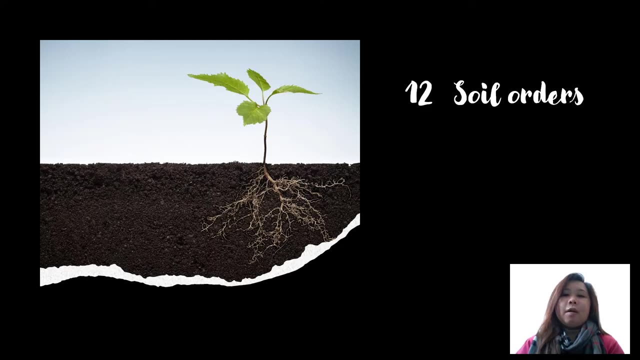 proceed now in discussing the 12 different soil orders. By the way, in this discussion we will only focus on discussing the different orders, the 12 orders, and under the soil orders, we will discuss the sub-orders. The 12 different soil orders are the following: We have anti-soil, incepti-soil, aridi-soil. 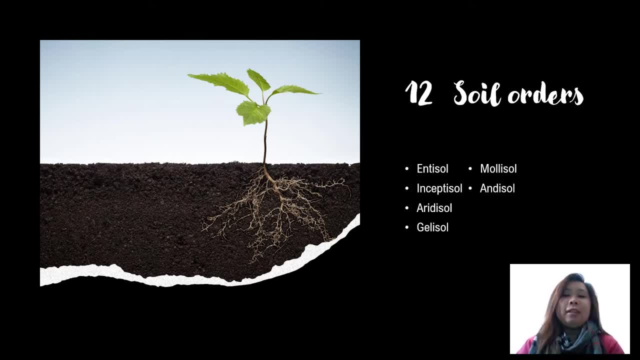 sali-soil, moly-soil, anti-soil, spod-soil, alfi-soil, poti-soil, oxi-soil, verti-soil and histo-soil. So let's discuss all of them. 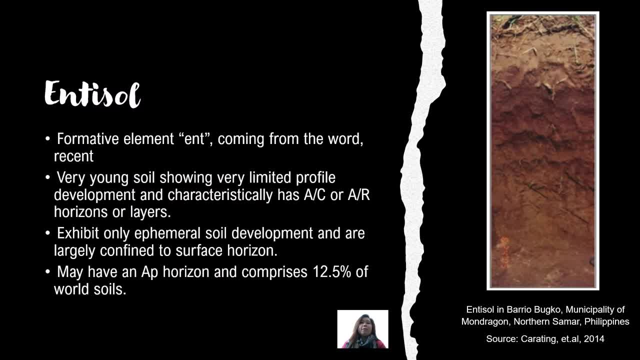 We have anti-soil as the first soil order. It has the formative element and, coming from the word recent, Anti-soils are very young soils showing very limited profile development and characteristically has the transitional horizons of A-C or A-R horizons or layers. 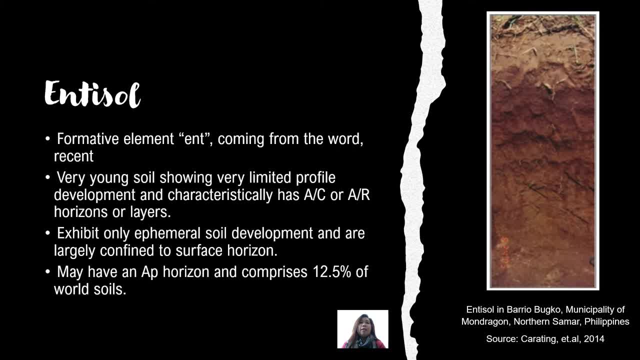 Meaning you only have the top soil and the bottom soil. So you only have the top soil and the bottom soil, So you only have the top soil and the parent material or the top soil and the bedrock. Anti-soils exhibit only ephemeral soil development and are largely confined to surface horizons. 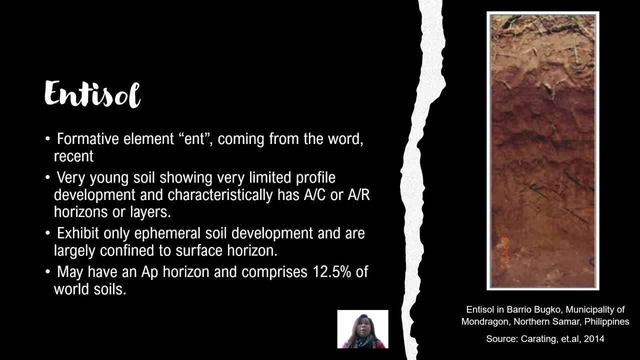 Anti-soil may have an A-P horizon, meaning a top soil that is being plowed, plowed regularly and comprises 12.5% of world soils. So an A-P horizon means a top soil that is being plowed regularly and comprises 12.5%. 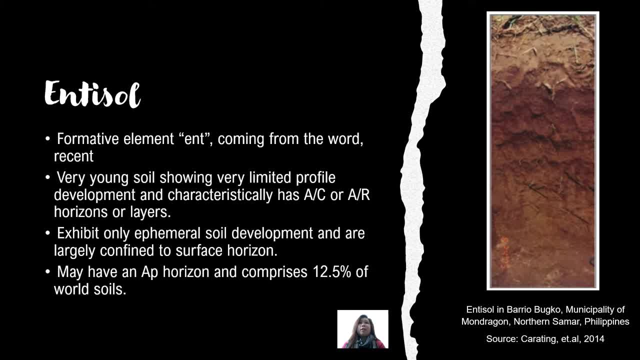 of world soils. So an A-P horizon means a top soil that is being plowed regularly and comprises 12.5% of world soils. So an example of anti-soil is in this photo. It is an anti-soil found in Barabugco Municipality of Mondragon, Northern Samar, Philippines. 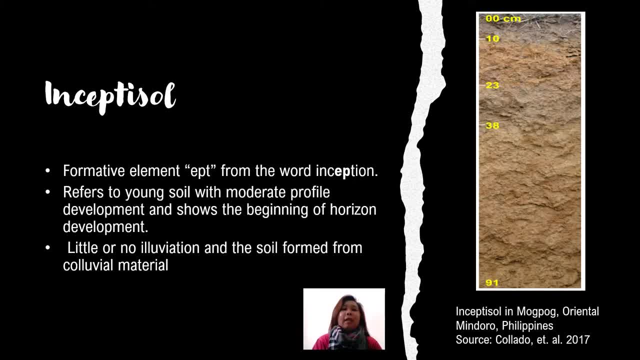 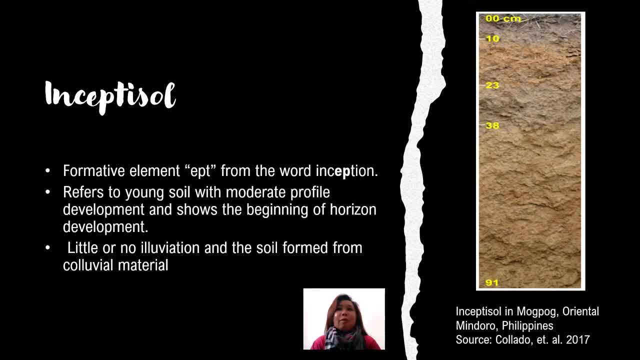 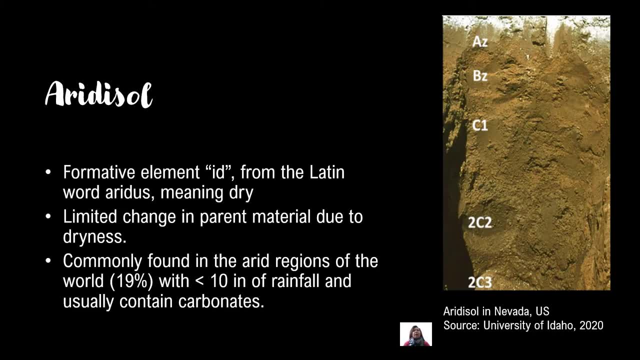 It refers to young soils with moderate profile development and shows the beginning of horizons. It refers to young soils with moderate profile development and shows the beginning of horizons, horizon or whatever horizon is present. Next we have is the aridisol: Aridisol. 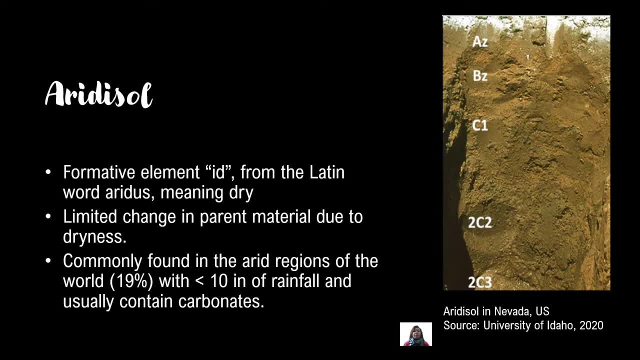 has a formative element, id from the Latin word aridus, meaning dry. There's limited change in parent material due to dryness and it is commonly found in the arid regions of the world- About 13 percent of the world with less than 10. 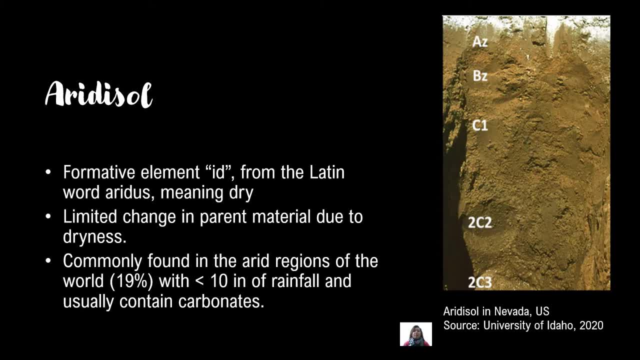 inches of rainfall and usually contain carbonates. This one is an example of aridisol found in Nevada, US. We don't have Aridisol here in the Philippines. The next one we have is the Jalisol. It has a formative element, id. When you have Aridisol by any given season, you need to. 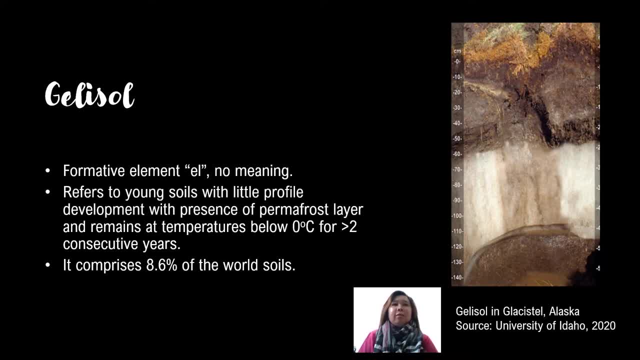 element L, and this refers to young soils with little profile development, with presence of permafrost layer, and remains at temperatures below zero degrees Celsius for greater than two consecutive years. it comprises 8.6% of the world soils, so a common example of jelly soil is found in Alaska. we don't have a 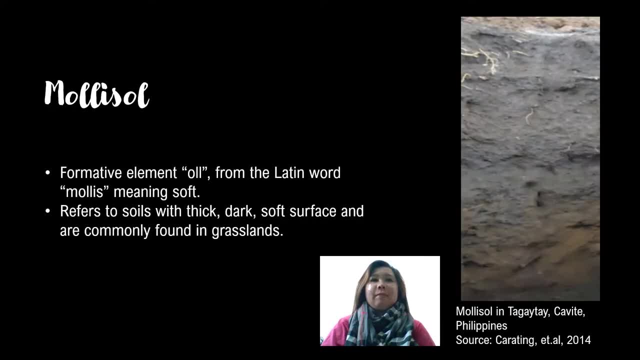 jelly soil here in the Philippines. next one you have is the molysool. it has a formative element all from the Latin word mollis, that means soft. this refers to soils with thick, dark, soft surface and are commonly found in the grasslands. example of molysoil is found. 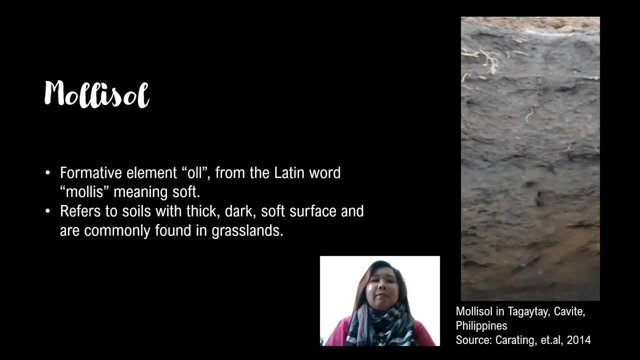 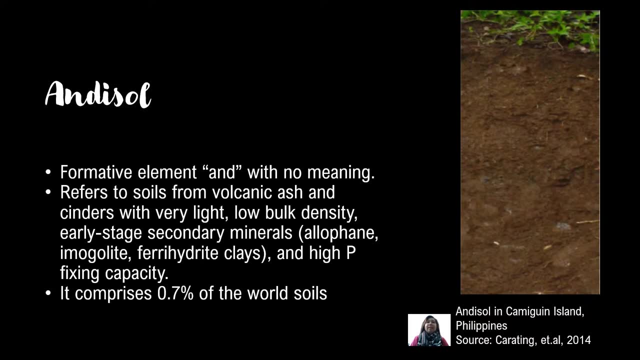 in Tagaytay, Cavite, Philippines. we also have antisol. It has a formative element and with no meaning. this refers to soils with volcanic ash and cinders with very light low bulk density and early-stage secondary minerals such as allophane imoveolite. 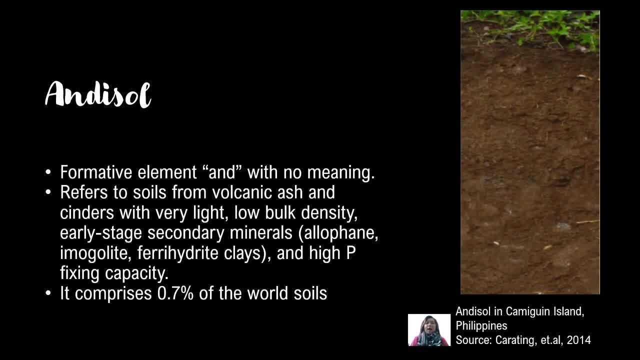 very high 될th place, and this soil are high in P fixation capacity, or phosphorus fixation capacity, and antis абсолют comprises 0.7 percent of the world's soils. this one is an anti-soul found in kamigin island, philippines. 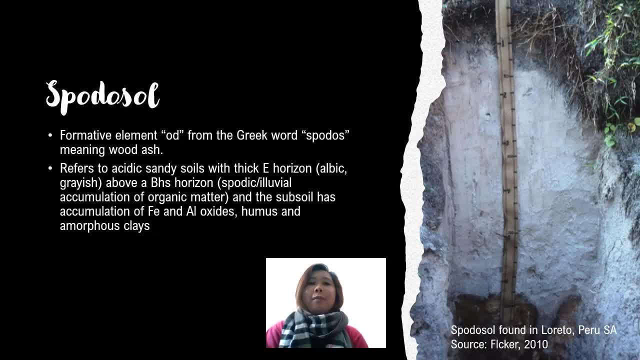 next one is spodosol. it has a formative element odd from the greek word spodos, meaning wood ash. this refers to acidic, sandy soils with deep e horizon: an albic or grayish horizon above a bhs horizon, or a spodic or alluvial accumulation of organic matter, as a subsoil has accumulation. 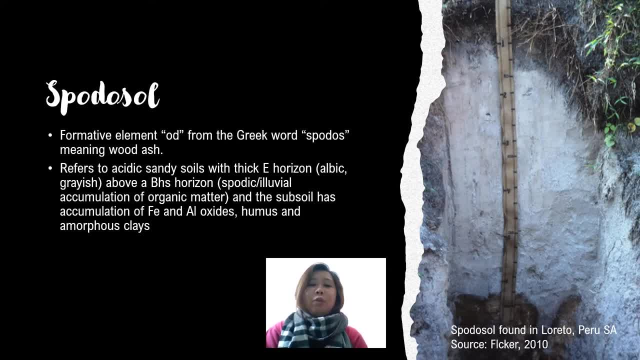 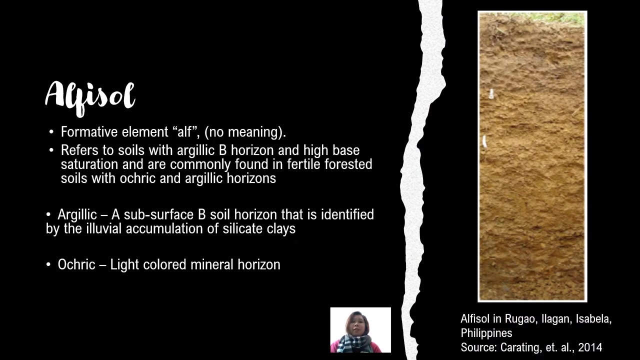 of iron and aluminum oxides, humus and amorphous clay. this one is a spodosol found in loretta, peru, southern america. next is alfisol. it has a formative element of, and this refers to soils with a gelic b horizon and high base saturation, and they are commonly found in fertile forested soils with ocric and. 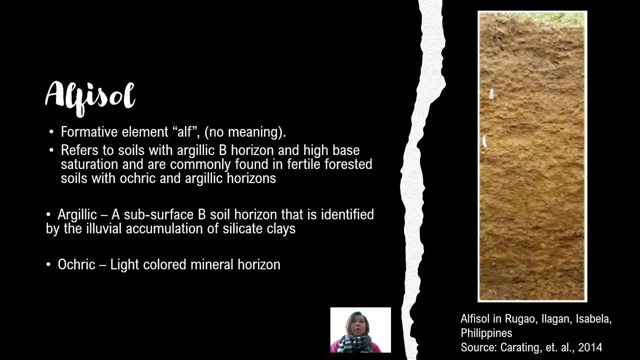 argillic horizons. by the way, argillic means it is a subsurface b soil horizon that is identified by the alluvial accumulation of silicate clays, while ocric is a light colored mineral horizon. argillic and ocric are both diagnostic. 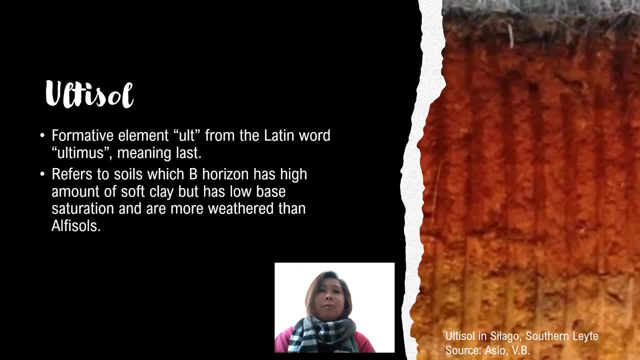 horizons. next is ultisol. it has a formative element old, from the latin word ultimus, meaning last. this refers to soil with b horizon that has high amount of soft clay but has low base saturation. weather than alphysols, they are usually acidic in nature. 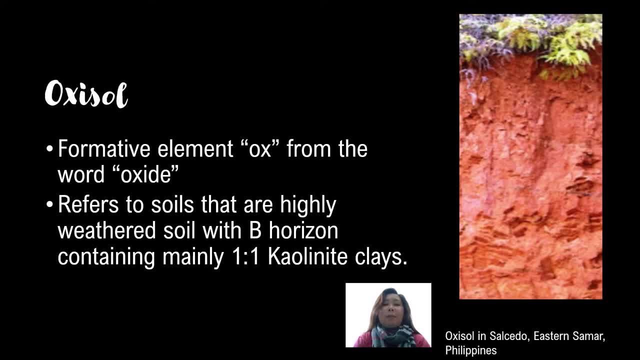 our next whole order is oxisol. it has a formative element, ox, from the word oxide. this refers to soils that are highly weathered, with b horizon containing mainly one is the one kd night place. an example of oxisol is found in salcedo. 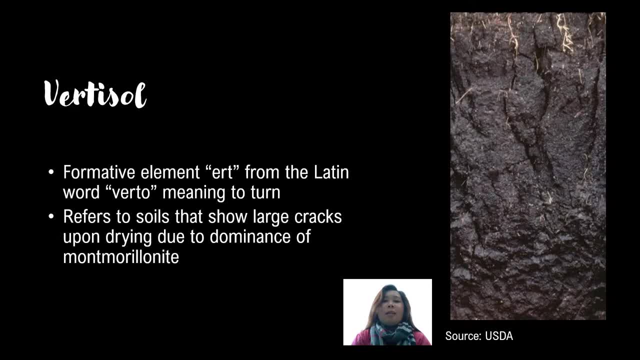 this turns summer in the philippines. the next one we have is the vertisol, that's a formative element, earth- from the latin word virto, meaning to turn. this refers to soils that show large cracks upon drawing due to dominance of mount marillionite. we all know that. 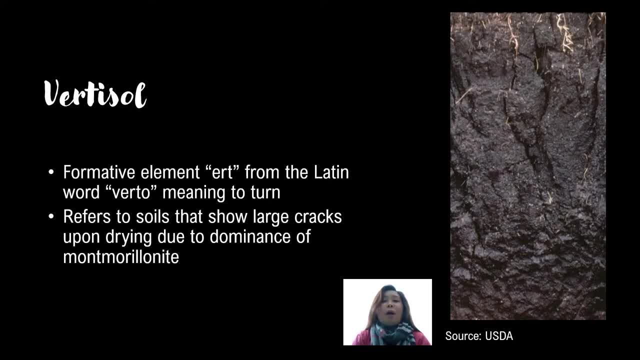 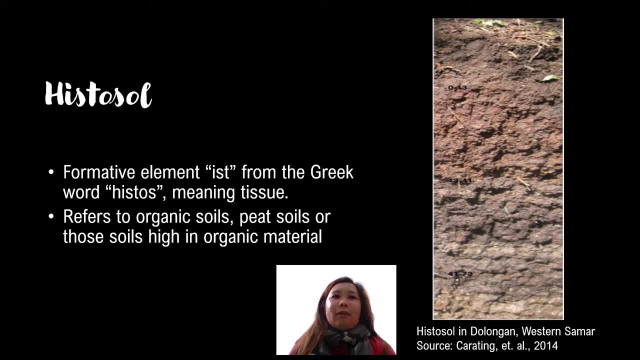 montmorillonite or montmorillonitic place, are prone to shrinking and swelling. our last soil, our, is histosol. it is the formative element is from the big word histos. that means tissue. this refers to organic soils such as peat soils or those soils with high 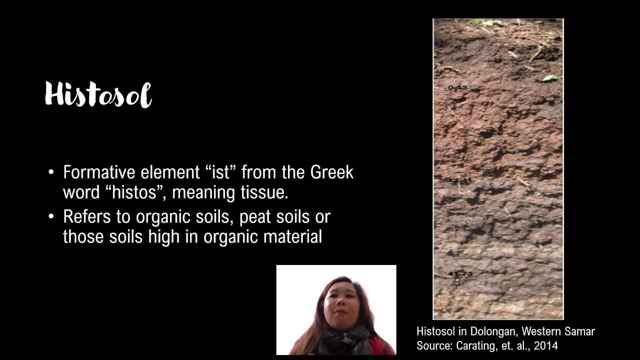 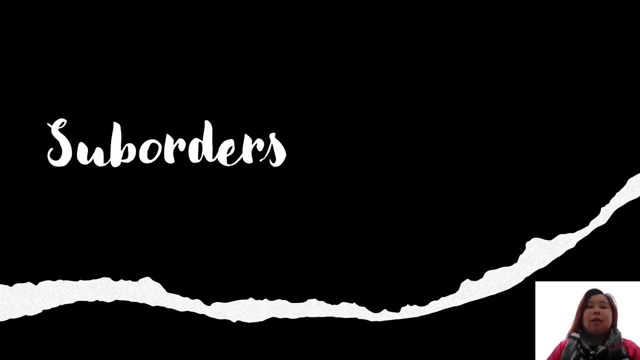 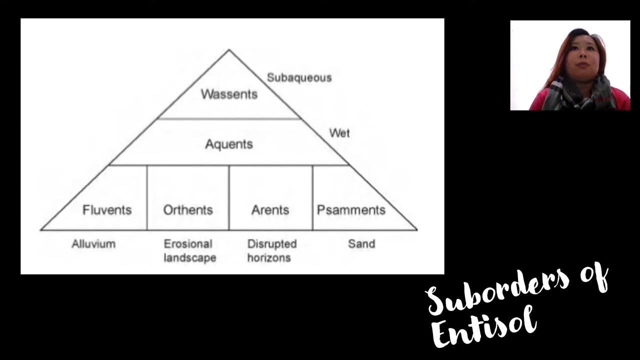 in organic material. in this example we have the histosol that is found in the longan western summer in the Philippines. now let us discuss the difference of orders. under the twelve orders in this triangle you can find the different suborders of antisol and emphasis is divided between permanent inundation by 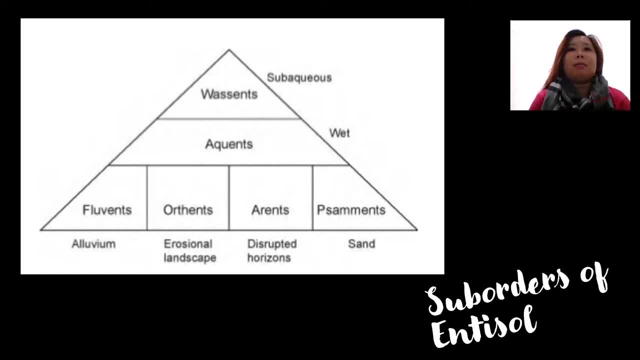 water, that is, the wassands, sub aqueous soils near surface saturation, which is the phase in that you can find that stage in Doppler mitad minus one frog child. so this is where you can compare these different seasonal geographic able to determine yours. allow for the plant grapes, both plant and 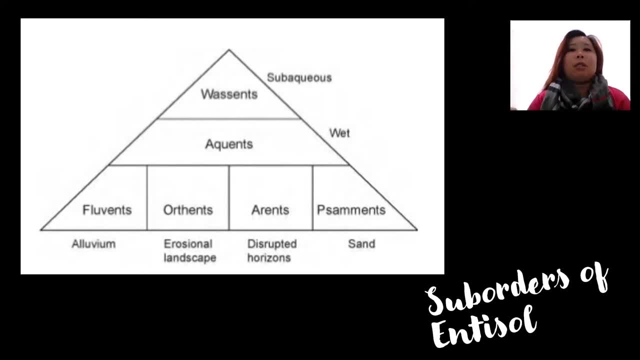 surface spiritually. we have to περιiao, specifically Northern. I'm in the West. it has to perform a lot. so now when we go to south Africa, in what Georgia we? we go to the north here, which is better to particularly 성 i like for at the 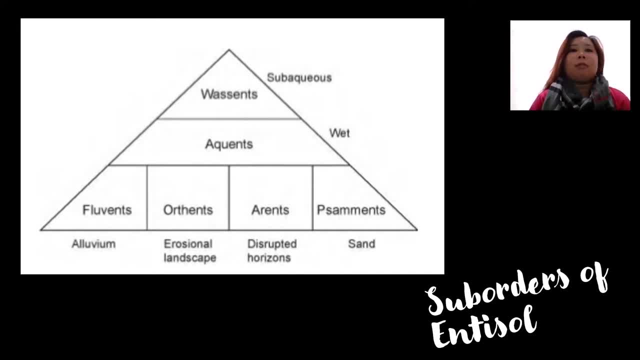 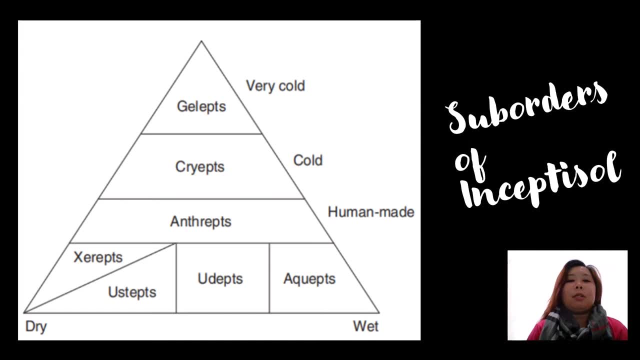 The irons which have disruptive horizons For the suborders of incepticel. we have the following: The aqueps, which has a water table at or near the surface for much of the year. Next we have the gelops. 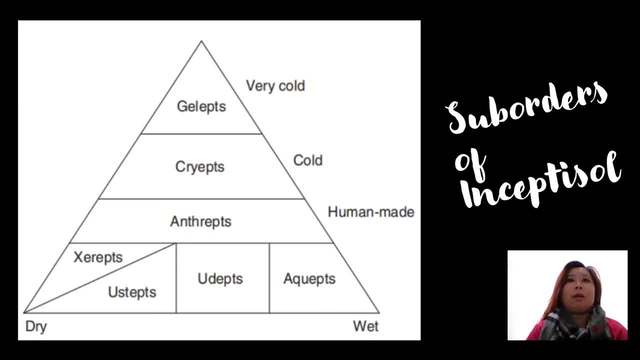 This gelops is common in very cold climates with an annual mean temperature of less than 0°C. For the cryops, these soils are common also in cold climates with an annual temperature between less than 0°C to 8°C. 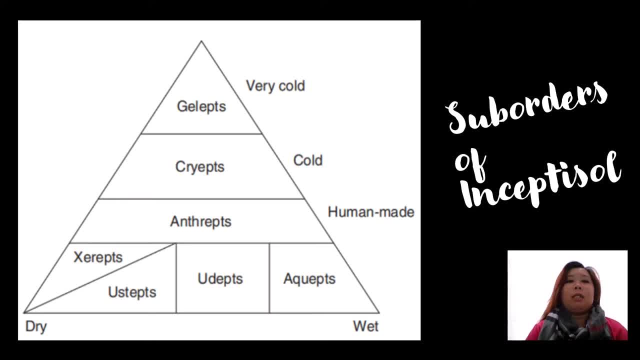 And then we have the oosteps. These soils are common in very cold climates, with an annual mean temperature of less than 0°C to 8°C. These soils are common in semi-arid and sub-humid climates. Next are the serops. 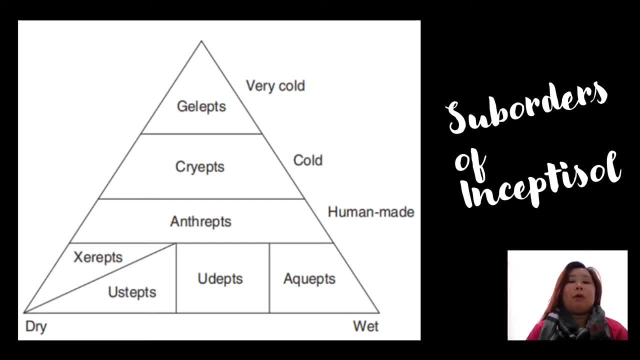 These soils are common in temperate, with very dry summer and moist winter climate. For the eudepts, these are common in areas with humid climates. And then we have the antreps, which contain markers of past agricultural Or past cultural habitats and anthropogenic or man-made activities. 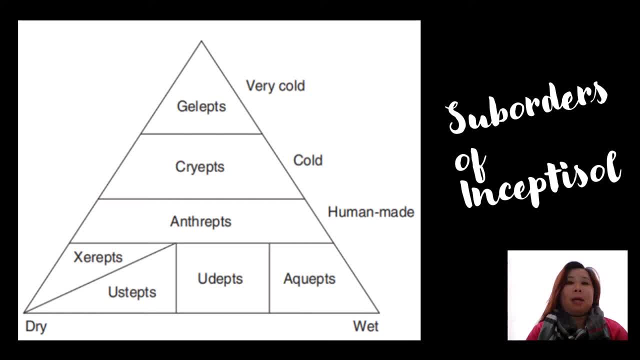 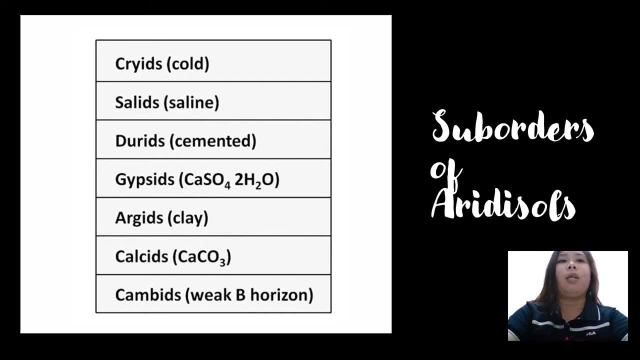 And these antreps can occur in any climate. Aridous soils have seven sub-orders, Namely: cryades, which have a cryic soil temperature regime. Salides, having a salic horizon within 100 cm of the soil. 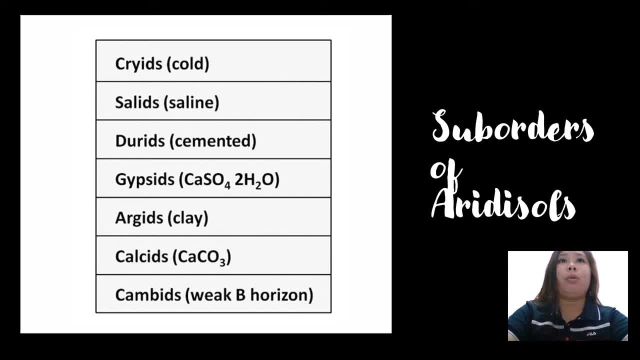 The reeds. these are soils that have a durapan within 100 cm of the soil surface. Gypsides are those that are having a gypsic or petrogypsic horizon within 100 cm of the soil surface And do not have a petroclastic horizon overlying the horizons. 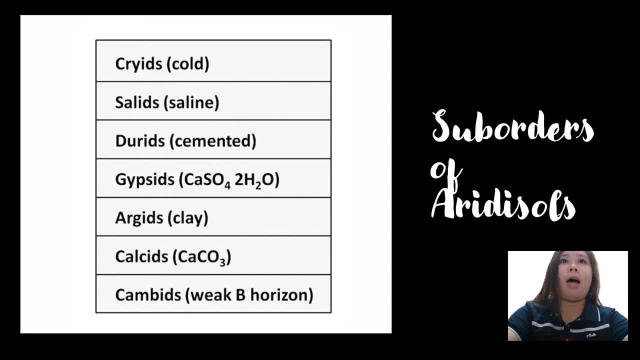 For the arid jades. these are soils that have a arid jade ornatic horizon And do not have a petroclastic horizon within 100 cm of the soil surface. Calcides are soils having a calcic or petroclastic horizon within 100 cm of the soil surface. 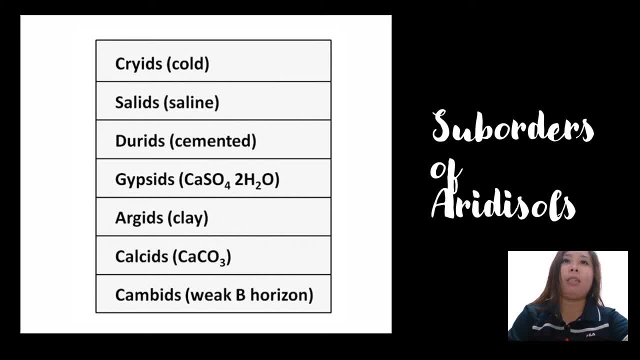 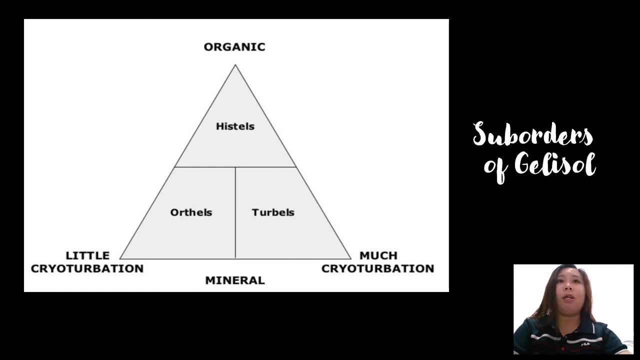 And last but not the least are the cambrides. These are soils that do not have the diagnostic properties defined in the other sub-orders. For the jelly soils, this soil order has only three sub-orders, Which are the following: Histos: those are organic soils similar to histosol. 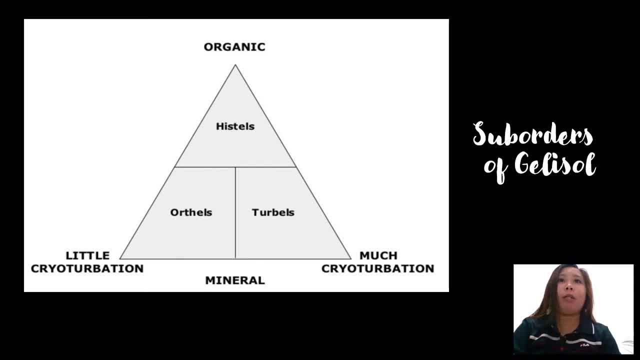 But 80% or more organic material from the soil surface to adapt a 50 cm layer or solid layer is found. Turbels is found over a one-third. horizons are broken or distorted due to cryoturbination And maybe ice wedges. 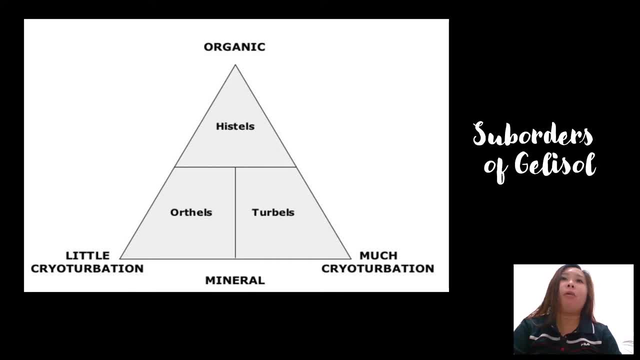 These are also common For all our tells. compared to turbels and his tells, it is dry compared to his tells and turbels and has little to no cryoturbation. By the way, cryoturbation means mixing of materials from various horizons of the soil. 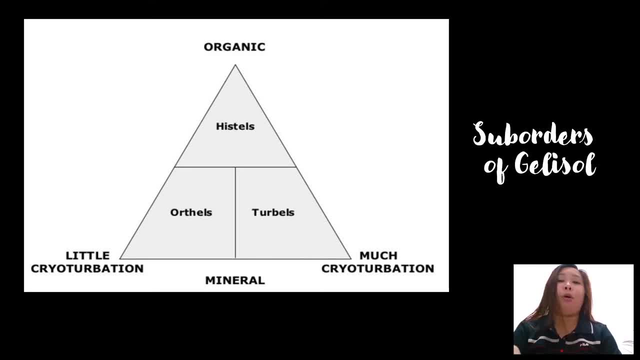 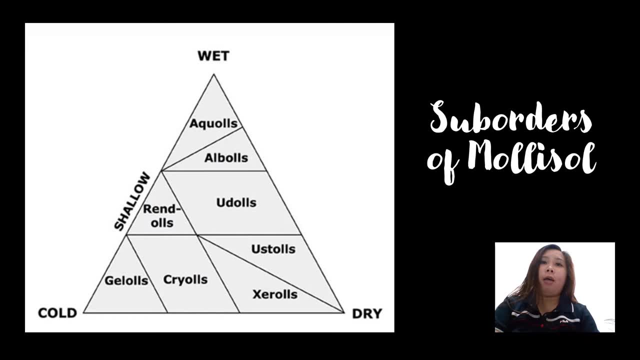 Down to the bedrock due to freezing and thawing. Next we have are the sub-orders of molysoin, And we have eight sub-orders for molysoin. Aquals are those soils that are wet, meaning wet molysoin. 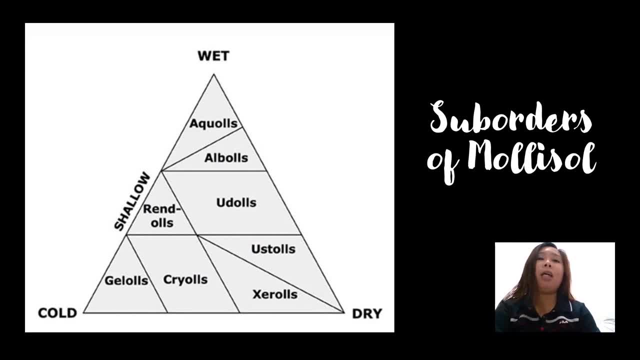 Albols: these are molysoins having albic horizons. Rendals: These are soils found in humid regions that formed in highly calcareous parent materials such as limestone, chalk and drift that is composed of mainly limestone or shell bars. 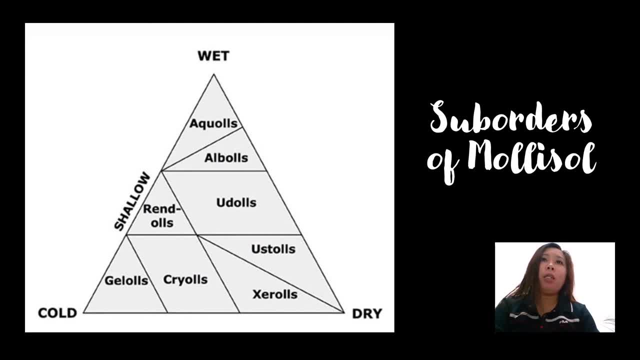 We also have the gembols. These are soils found in cold regions. For cryols. these are deep, freely drained, with a correct temperature regime. molysoin Cerols are those soils having a steric soil moisture regime. 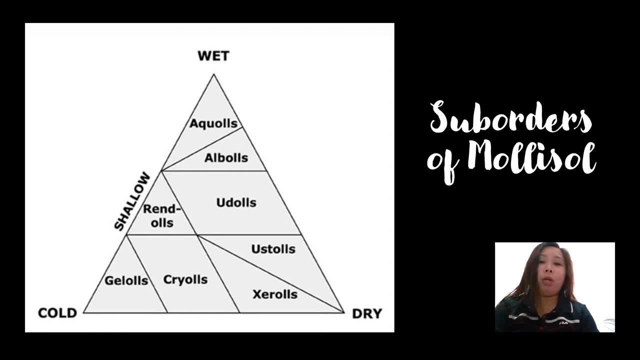 Ustols are those that are freely drained and commonly found semi-arid to solve humid climates with ustic soil moisture regime. And that's about the list Or the udols. These are soils that are more or less freely drained And are commonly found in humid regions. 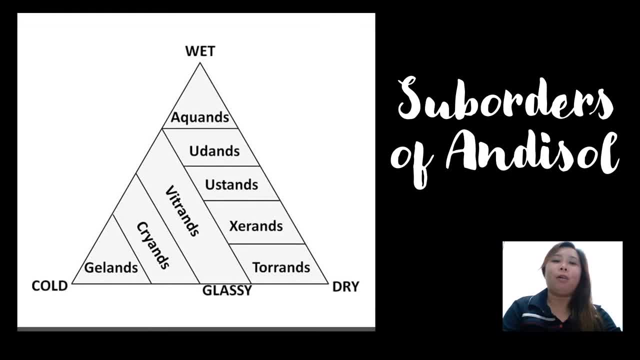 The next are the sub-orders of andesol. There are eight sub-orders of andesol. First we have is the aquand, or aquans. Aquans have a histic epipedon or have aqueous conditions in a layer at a depth of 40 to 50 centimeters. 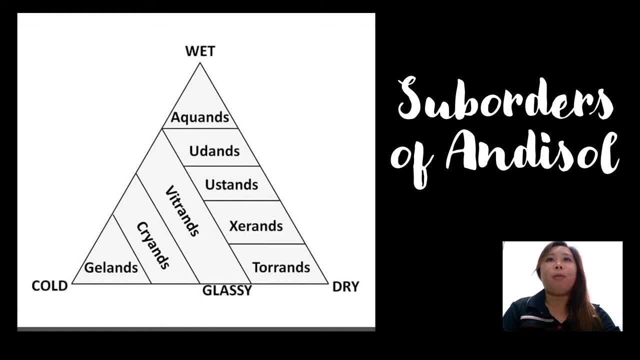 Below the mineral soil or from the top of an organic layer For the cryans. Cryans are those soils that have cryic soil temperature regimes. For gelands, These are soils having a gelic soil temperature regime, Meaning the mid-annual soil temperature is less than 0°C. 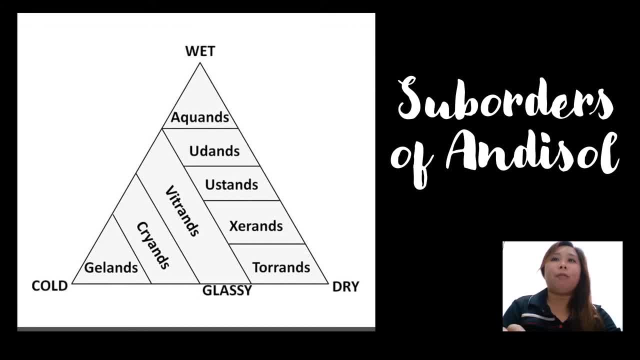 Under the sub-order of andesol is the torrent or the torrent. Torrents have aridic soil moisture regimes, Ustans. These soils occur in tropical regions that have ustic moisture regimes characterized by extended dry periods. Udans have humid climates. 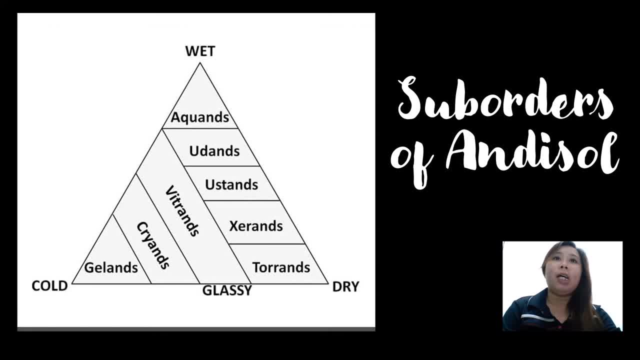 And a relatively high content of water, Healthy type B for plants to use And with trends. Those are soils that are well-drained, That are coarse textured And are dominated by glass. And last but not the least, Are the sirens. 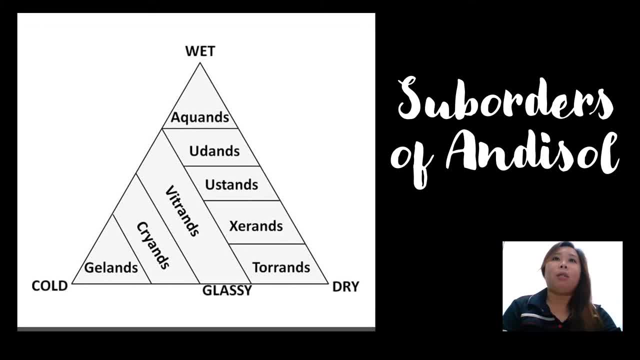 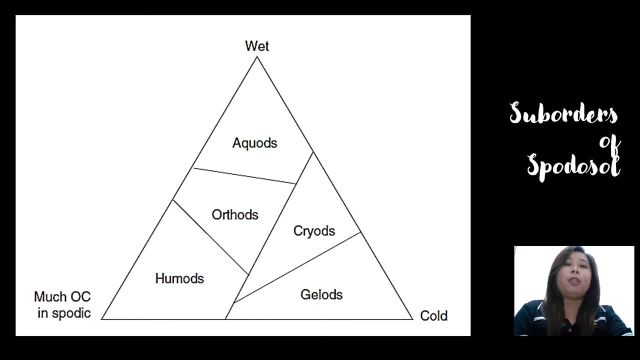 These soils are found in warm And Closed areas having dry summer And cold and moist winters. Next we have are the sub-orders of spodosol For the aquods. Aquods are spodosols having aquiconditions within 50 cm of the mineral soil surface in most years. 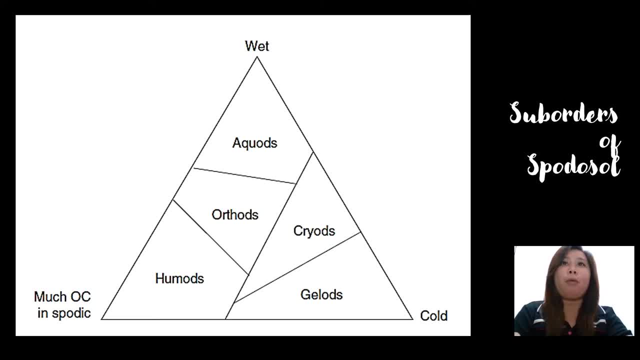 And have a heistic epipedon or redoximorphic features In the upper 50 cm. We also have the gelods. These are soils that are better drained And have gelic soil temperature regimes And are common in areas with high latitudes and altitudes. 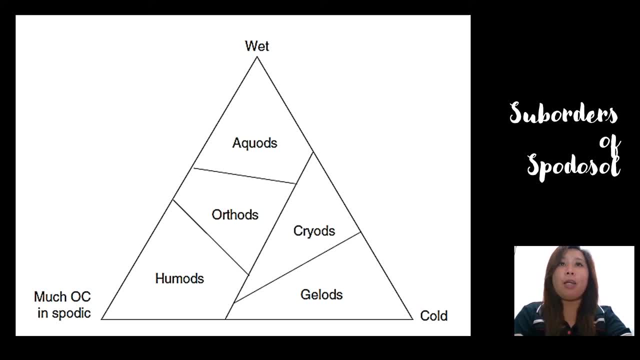 And then we have the cryodes. These are soils having cryo, Cryo temperature regimes And are common in Lower altitudes And latitudes Than the gelods. And then Eumods Or eumods. These are not as poorly drained as aquods. 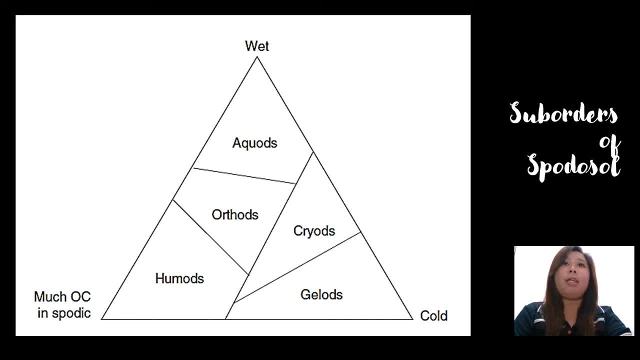 And have spodic horizons containing 6% or more Organic carbon. And then we have the orthods, The last one. These are soils that are better drained With spodic horizons And have spodic horizons containing less than 6% carbon. 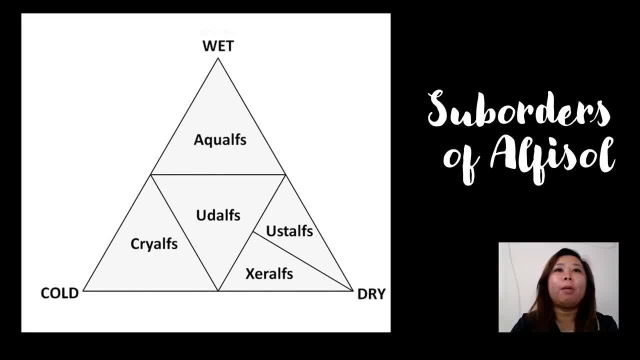 For the alfie soils We have five sub-orders. First we have are the aqualps. Aqualps have aqueous conditions For some time. in most years, Within 50 cm of the mineral soil surface Have redoximorphic features. 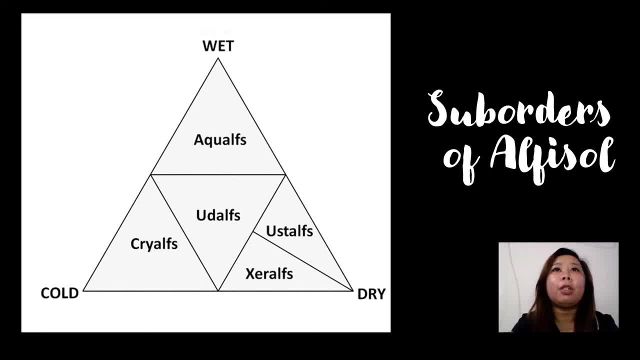 And usually Occupying depression areas Or Low gradient landscape Subject to seasonal Inundation Or high water tables, And then for cryo, These soils have Cryic Or isofligid Meaning. The annual temperature is 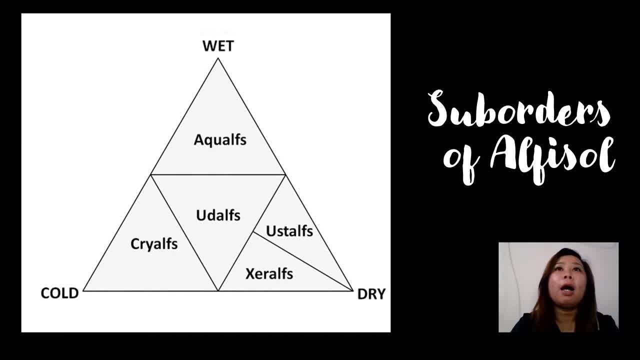 Less than 80°C Isofrigid Or cryic temperature regime And we have oostalps. Oostalps have, From name itself, Have oostic soil moisture regime, Meaning The soil moisture is limited But available. 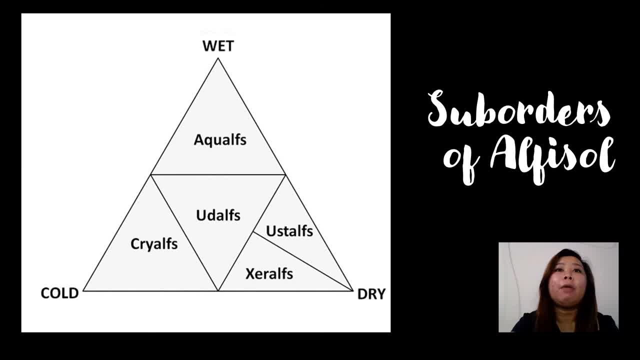 During the portions Of the growing season. Then we have the serops. From the name itself, It has Or it has. Those soils have Seric soil moisture regime, Meaning It is moist And cool In winter And warm and dry. 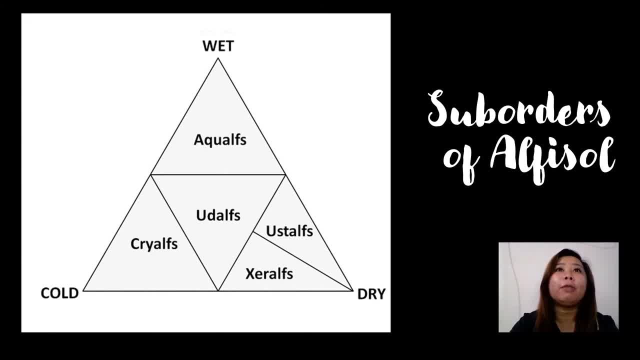 In summer. And then The eudulfs. Last but not the least, Eudulfs are those soils Having Well distributed rainfall, But Not as wet As the aqua, Nor as cold As the cryo. 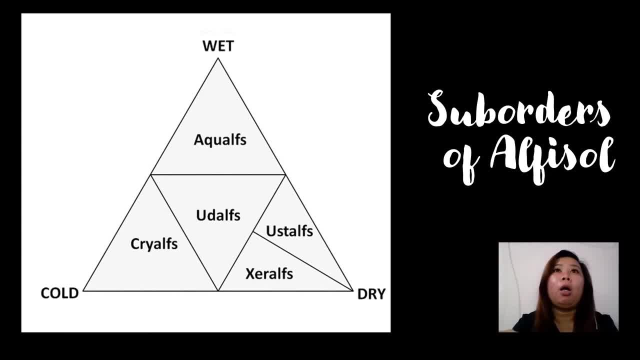 And have Eudic Soil moisture regime. By the way, Eudic means The soil have enough rain Or the area have enough rain In summer, So that the amount Of storm moisture Plus rainfall Is just equal. 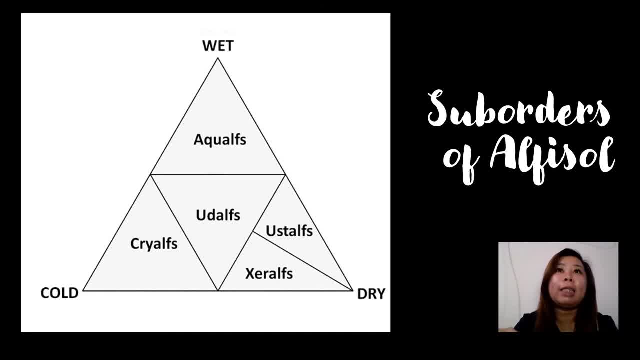 To Or exceeds The amount of Evapotranspiration And Isofrigid. It means that The soil, The area Where the soil Has mean Annual Soil temperature Of greater than Zero degrees celsius. 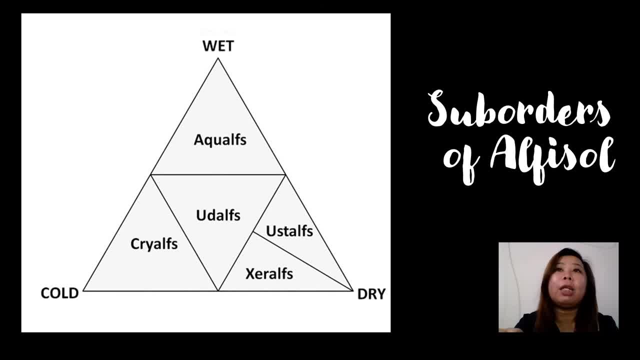 But less than Eight degrees celsius, With A difference between Mean summer And mean winter Soil temperature Of less than Five degrees celsius And less than Eight degrees celsius, With A difference between Less than 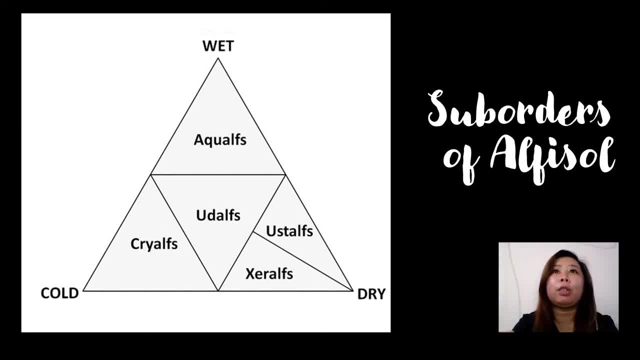 Five degrees celsius At Fifty centimeters Below the surface, And Warm Summer Temperatures. So Moving on With The suborders Of Eutisols, Eutisols Have One. 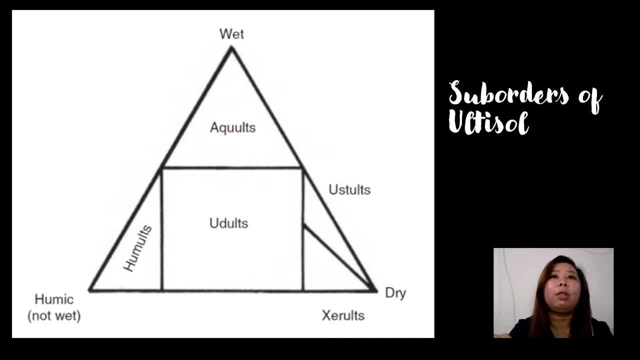 Two, Three, Four, Five Suborders. First Are The aquilts. So Aquilts Are Saturated With Water At Some Period During A normal Year, Or Artificially. 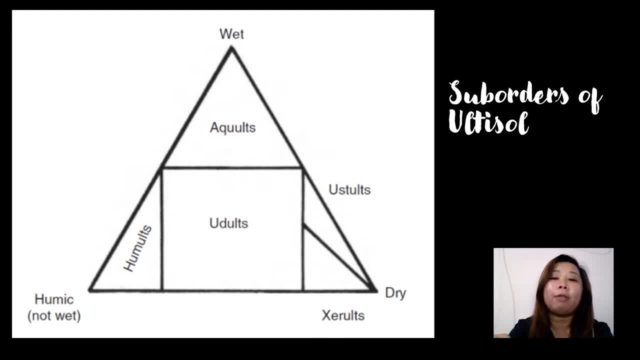 Drained Aquilts Have Redoxomorphic Features In All Layers Below Twenty-five Centimeters Or Any Api Horizon Of Present And Plants What Do Not. 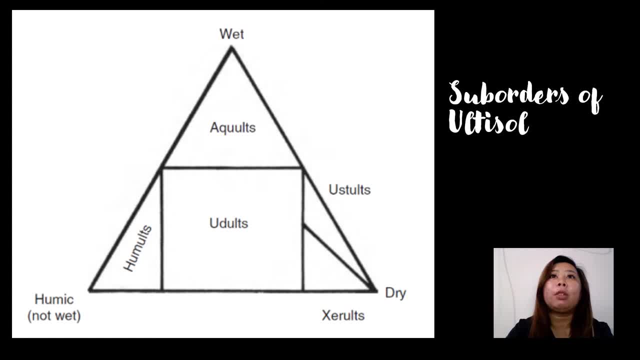 Have Characteristics Of Wetness Specified In The Aquilts. So Eumolds Contain More Than 0.9% Organic Carbon In The Upper 15,. 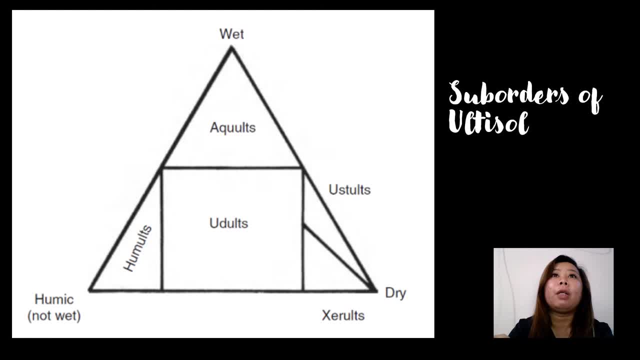 Centimeters Of The Arginic Or Soil Moisture Regime. By The Periodic Means There Is Extremely Wet Moisture Regime, The Dry Periods Of 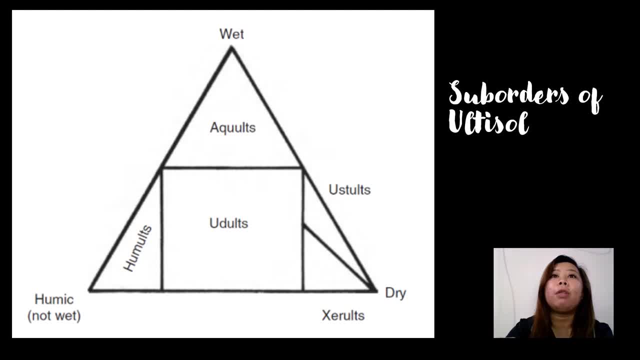 These Soils Are Of Short Duration And Organic Carbon Contents Are Lower. Seasonally Available In Etiquette Amounts For At Least One Scrap Per. 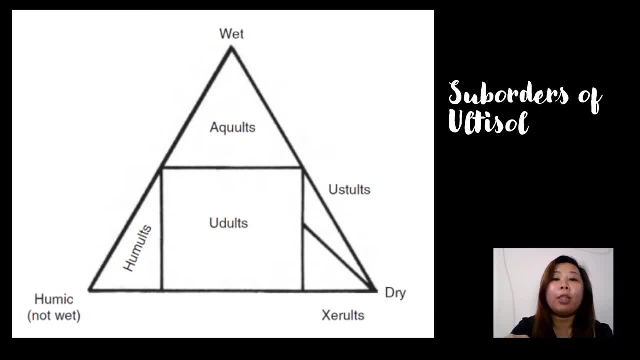 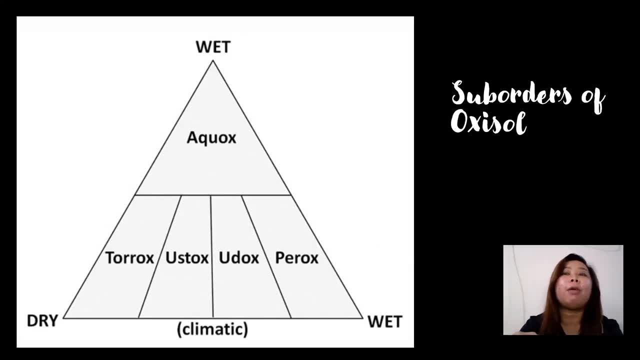 Year, And Then The Sorrelts. Sorrelts Are Common In Areas Of Extremely Dry Summers And Moist Winters, And Water, With Water Table At. 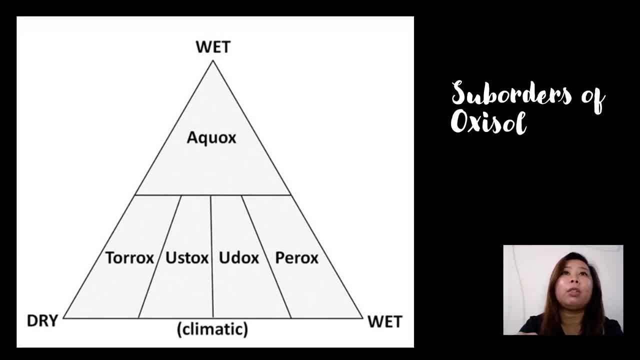 Or Near The Surface For Much Of The Year, And Then The Tall Rocks. These Are Common In Arid Climates. Woodstocks Are Common In 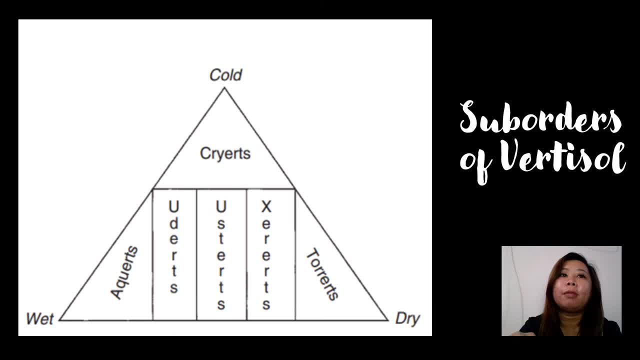 And Then We Have The Suborders Of Verticals. Again, We Have The Upwards With Acid Conditions For Some Time In Most Years, And Have 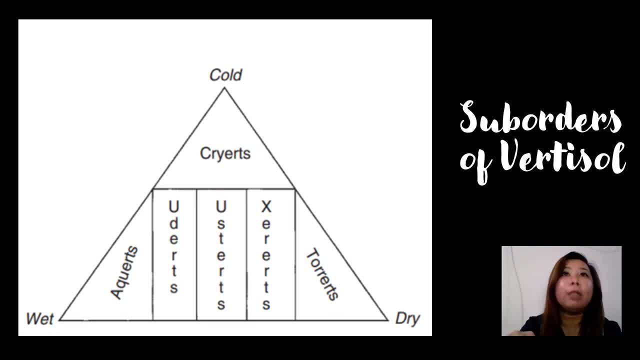 Presence Of Redoxomorphic Features, And Then Our Frigid Salt Temperature Regime And, Unless Irrigated, Have Cracks That Are Open At Least Sixty. 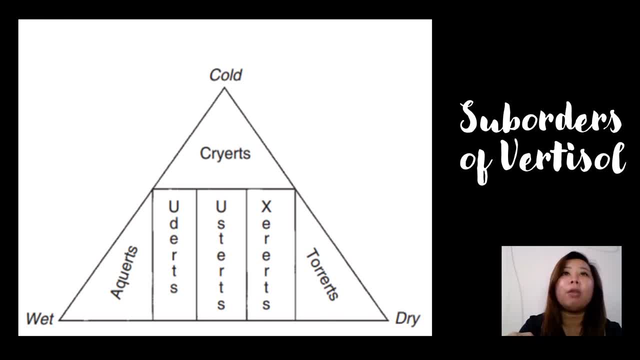 Consecutive Days During Summer, But Are Closed At Least Sixty Consecutive Days During Summer. And Then We Have Cracks That Are Open Less Than 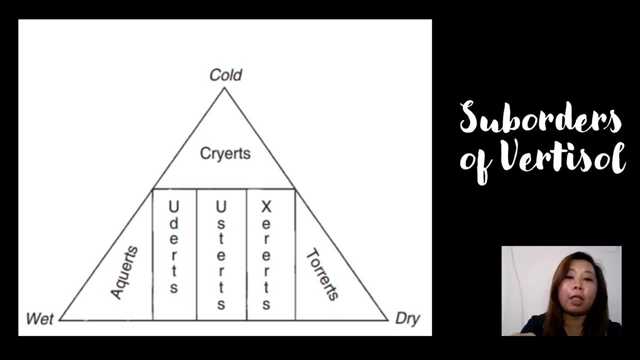 Sixty Consecutive Days During Summer, And Then We Have Cracks That Are Open Less Than Sixty Consecutive Days During Summer. So If You